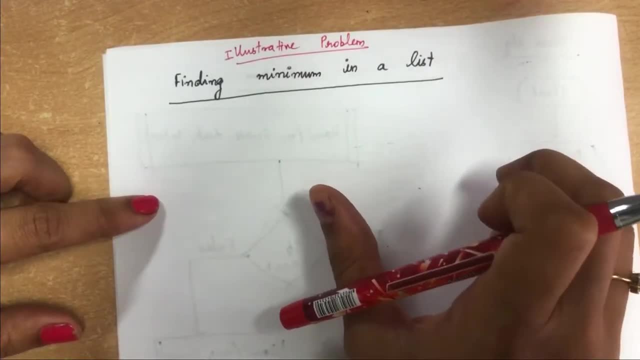 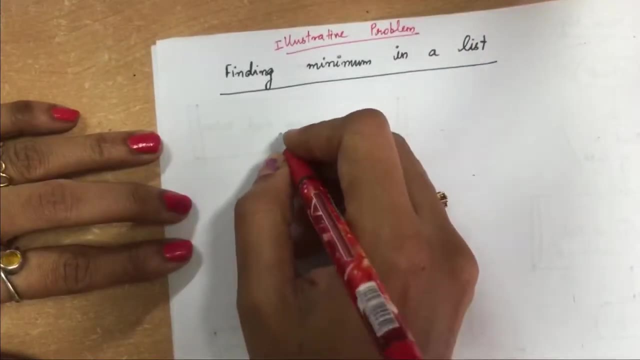 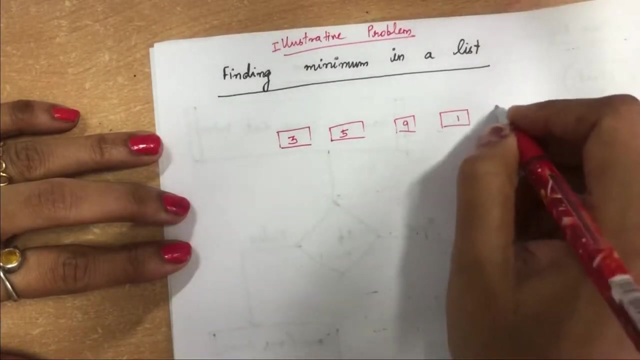 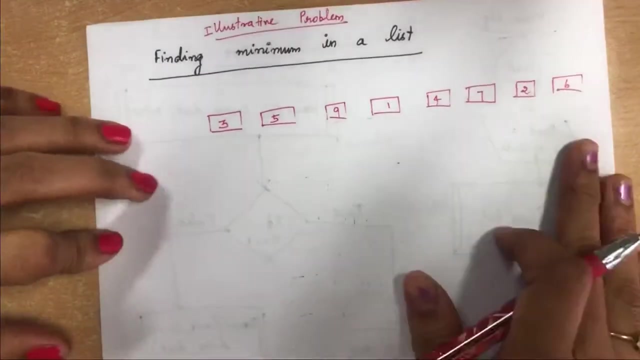 will be given. You have to find out the minimum numbers in the list. This is the problem which has been given. So for this I have to write the algorithm and flow chart. So visualize, suppose, if I have a numbers like this: 3, 5,, 9,, 1,, 4,, 7,, 2 and 6.. So these are the numbers which I have. 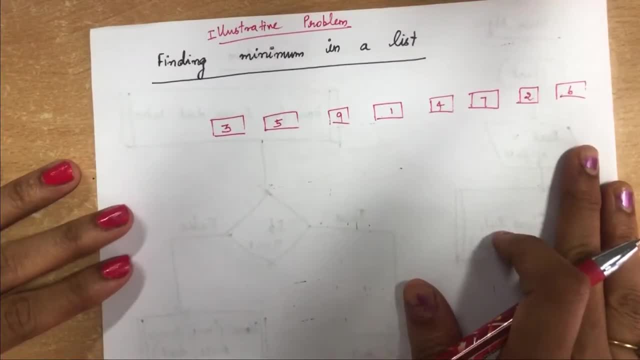 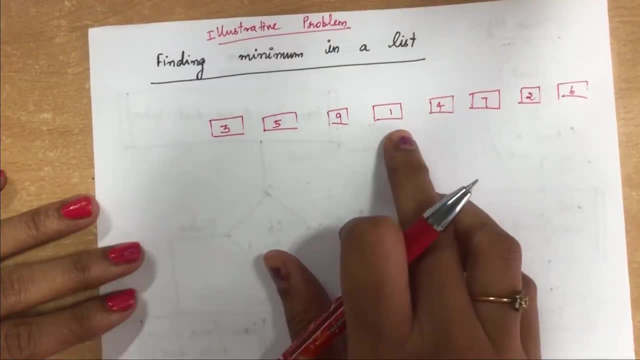 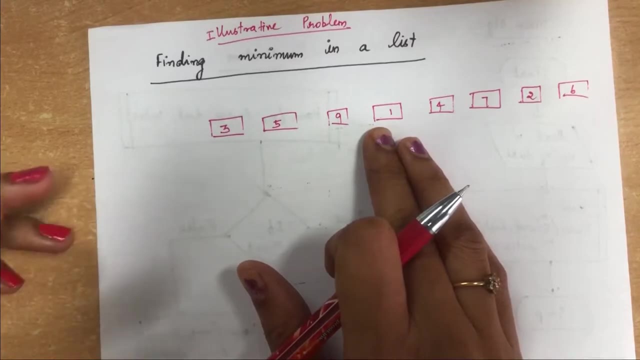 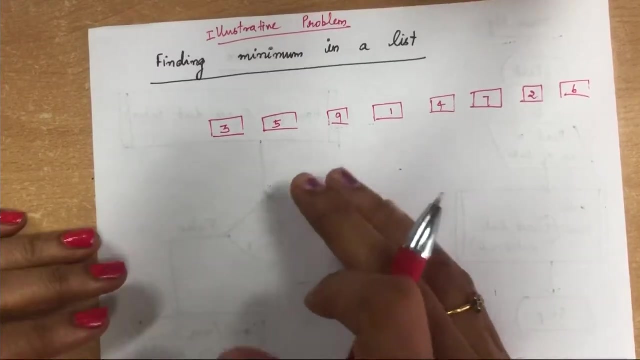 tell that 1 is the smallest among all the numbers. So minimum number in the list is 1.. But if the same problem, if it is to be done by the computer, it has to do some process. If you are going to do with the help of a problem program, then some set of procedures has to be followed. That is what 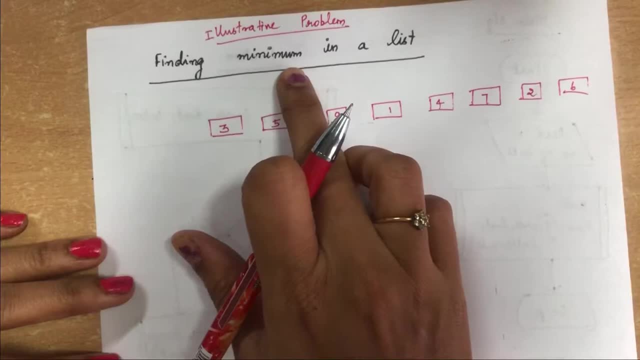 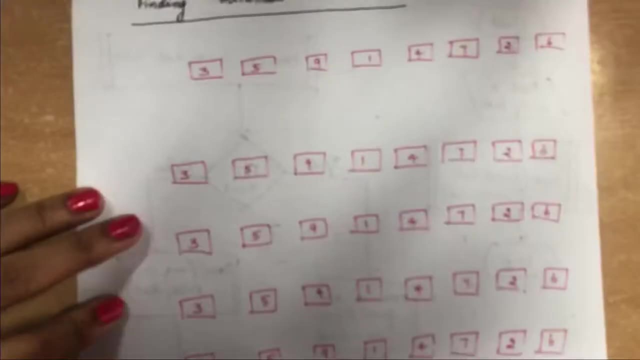 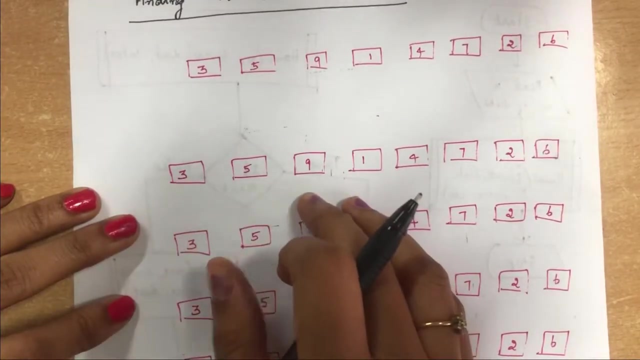 we are going to see in this, So we are going to find out the minimum number in a list. So when a simple set of functions has to be taken one by one, two by one, three by one, three by one, five by one and six by one, that is, set of environment and 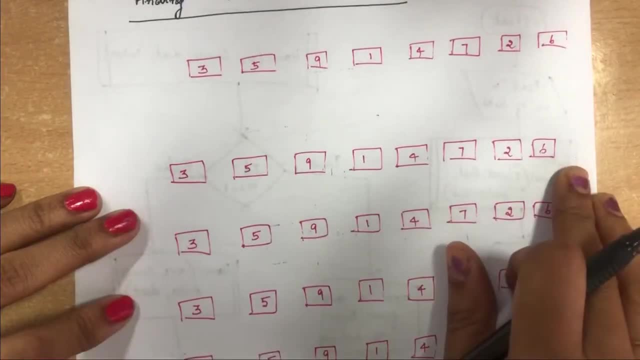 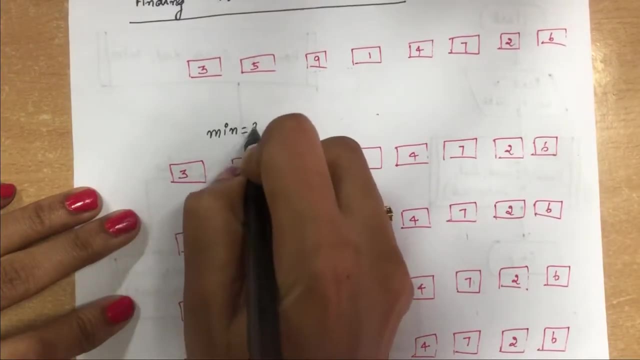 the number, that will you to find out the entire or the thousand unit unit number. OK, now we will see the step-by-step procedure for finding home the minimum number in a list of numbers. So here: 3,, 5,, 9,, 1,, 4,, 7,, 2, 6, this is a set of numbers which I have f. 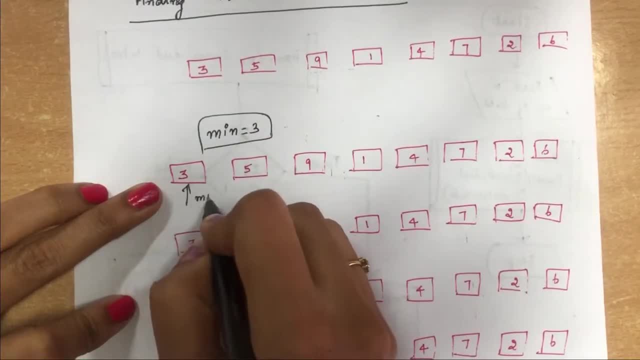 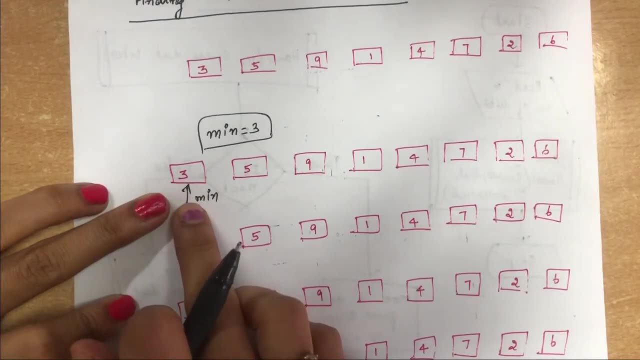 10. 6. friendships. So this is the minimum number. First I will set the minimum number to be the first element. So the program does not know which is the minimum number. So first what I have to do is I have to set this minimum number to be minimum. that variable value stores this, the first element in the list. 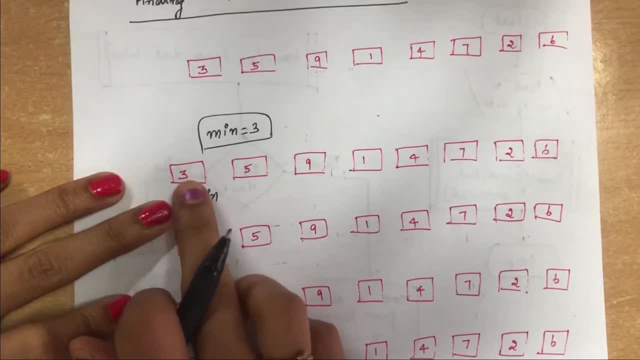 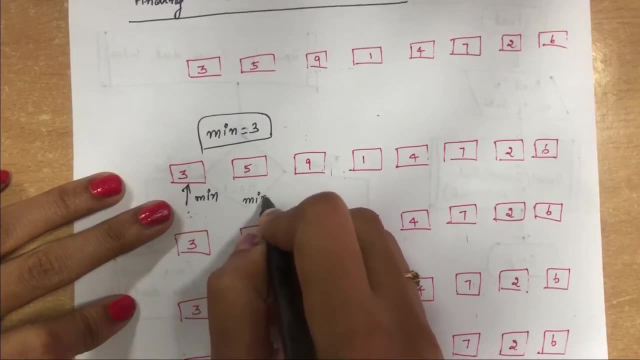 that is min. Now what I have to do is I have to compare this number with the next element in the list. One by one, I have to compare. So the first step is that I will be comparing whether minimum is greater than the next element, that is, 5.. So what is minimum value? that is 3.. 3 is greater. 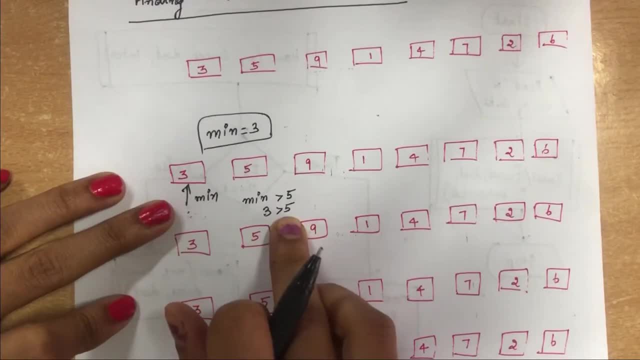 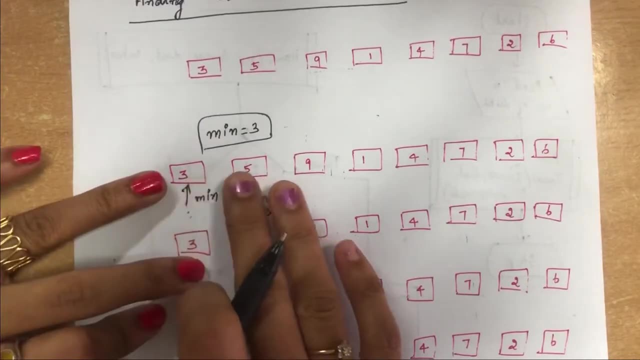 than 5.. Whether 3 is greater than 5.. No, it is. no, it is not greater, So it will go to the this. there is no change in exchanging the elements. When you compare 3 and 5,, 3 will be in this place and 5. 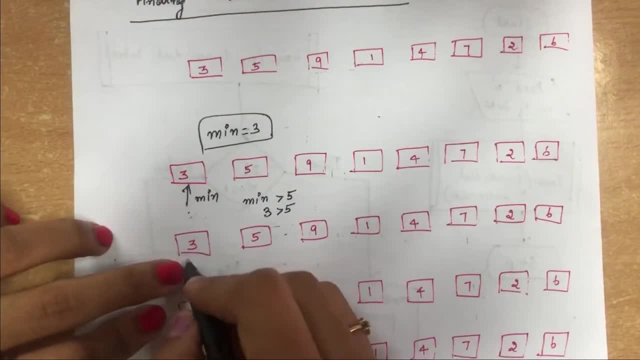 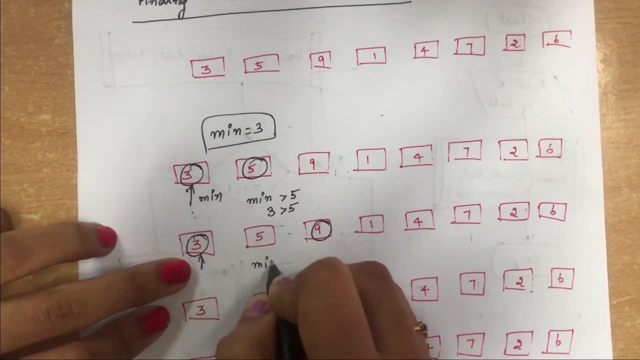 will be in this place. Now what I have to do is I have to compare this: 3 with 3 with 9.. Okay, 3 with 9.. So, again, I will check whether minimum value is greater than this 9.. So what is minimum value? 3 I have 3 is greater than 9.. No, So there. 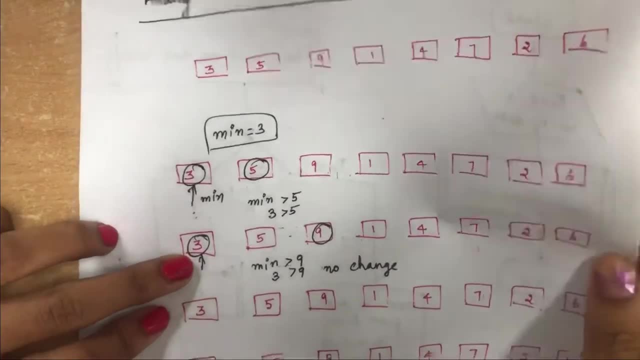 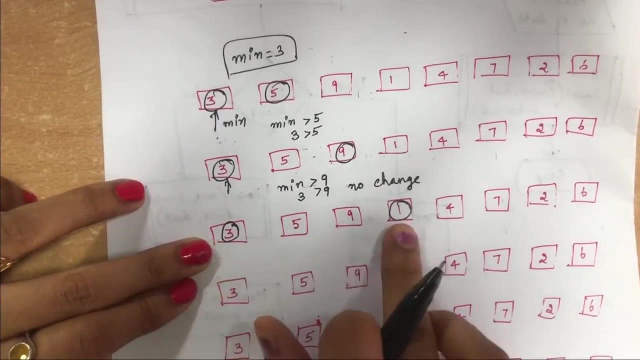 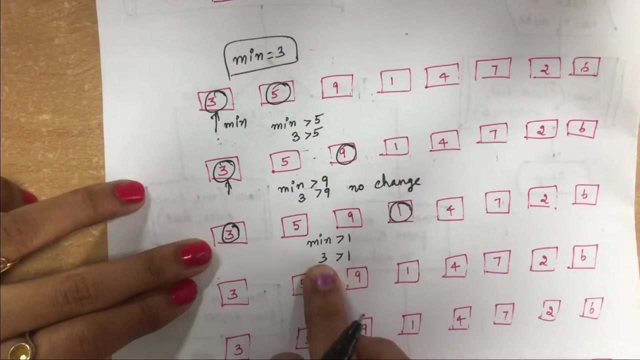 is no change. Okay, it is. no, it is not greater. So there is no change. So now what happens is I have to compare this 3 with 1.. So when I am comparing 3 with 1, minimum value is greater than this 1. Minimum value is 3.. Yes, it is greater. 3 is greater than 1.. So what happens? 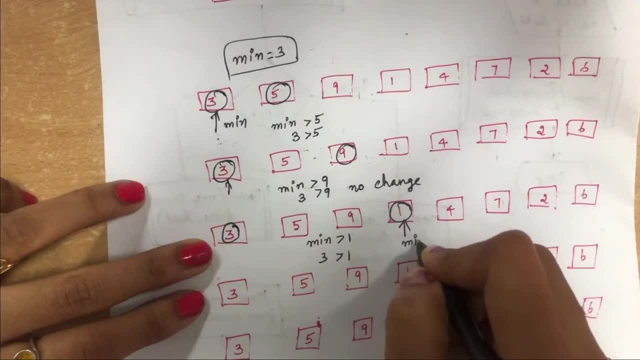 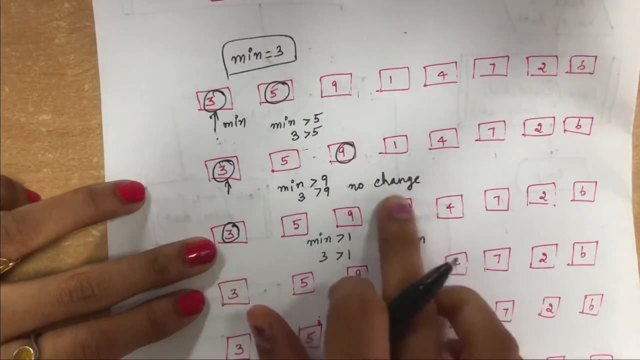 is that I have to set this as the minimum value. When this condition satisfies, then I have to set this 3 minimum value to be this the new value. So now this is the minimum value. What I have to do in the next step is I have to compare. 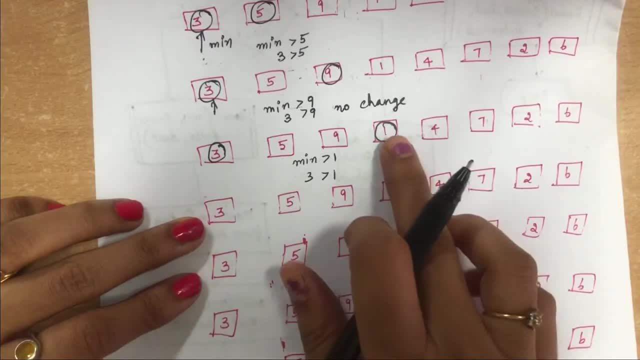 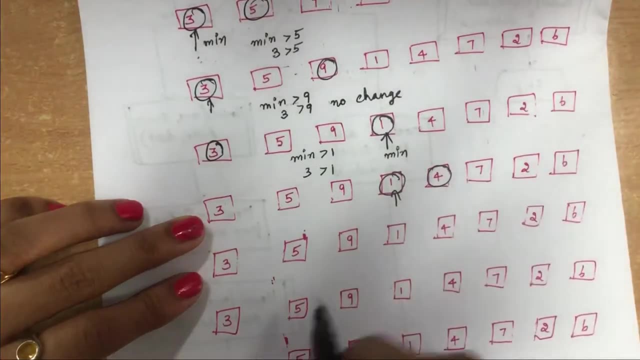 already I have compared all these 3,, 5,, 9.. So I have to compare this 1 with the next number in the list. So 1 will be compared with 4.. 1 will be compared with 4. That is, 1 is minimum value. 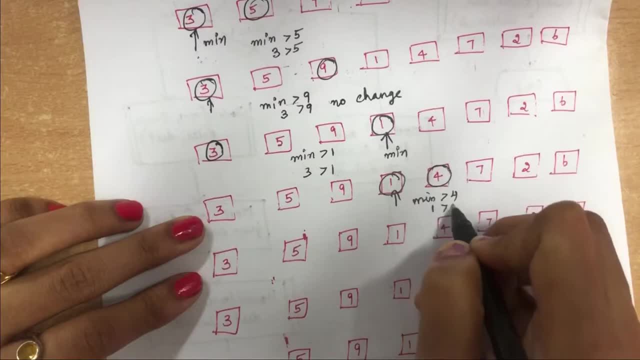 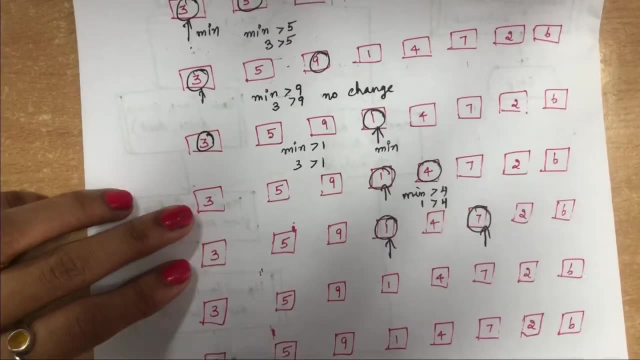 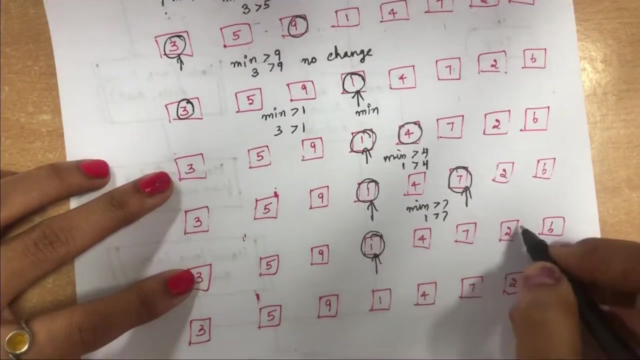 That is, it minimum is greater than 4.. That is, 1 is greater 4. no, it is not greater. so it now it checks. this one value is compared with 7. again, this minimum value is greater than 7. 1 is greater than 7. no, so again, what happens is in the next step. 1 is: 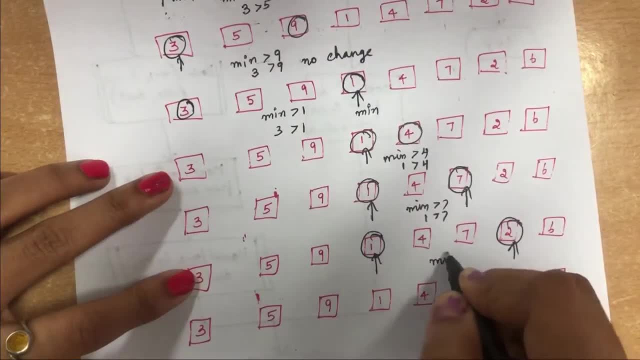 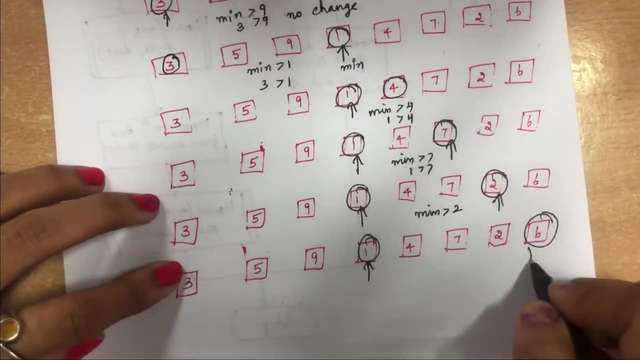 compared with 2, so there is no change. so minimum value is greater than 2, so there is no change. so now this 1 is compared with the last element of the list. so again, also the 1 is greater than 6. no, so there is no change. so when this is the case. so what happens is when you finish find: 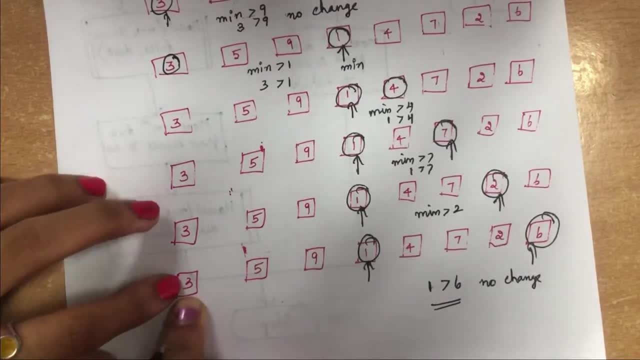 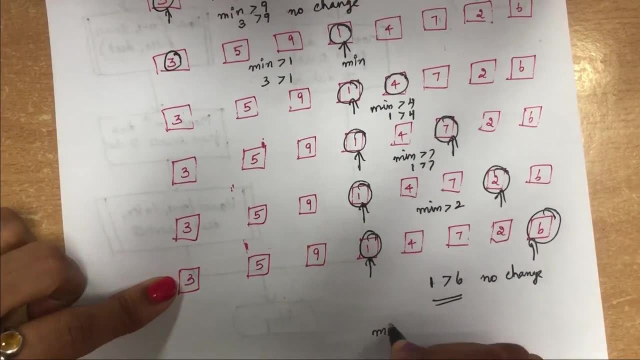 traversing all the elements in the list, you you have traversed, starting from first number and you have traversed till the last number in the list. so, once you have completed, so what is the minimum value which you are having which is stored now? now, the minimum value stored is 1, so this is: 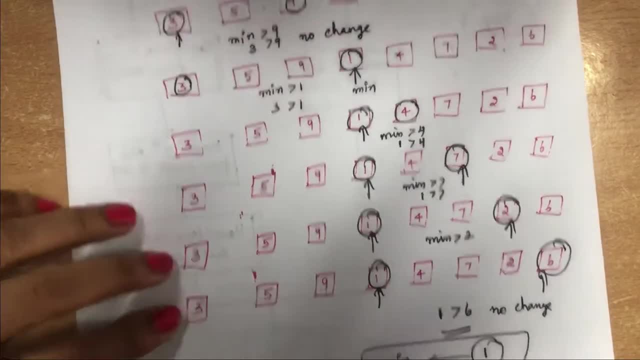 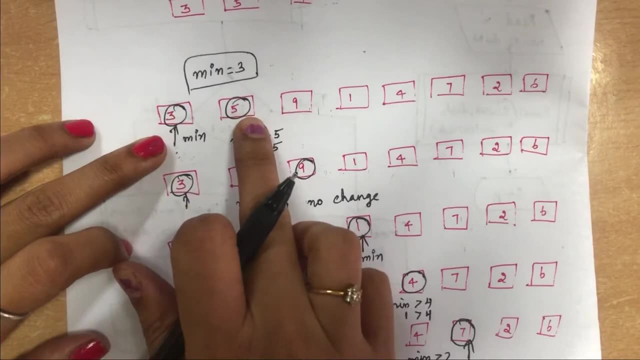 an output. this is how you have to find out the answer. so what i have to do is, first, i have to set this minimum value and i have to compare whether this 3 is compared with 5. so when this condition, when this condition satisfies, then i have to. when this is greater, then i have to set the second value as minimum. 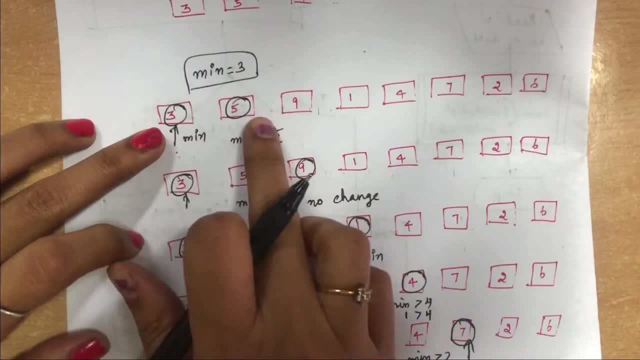 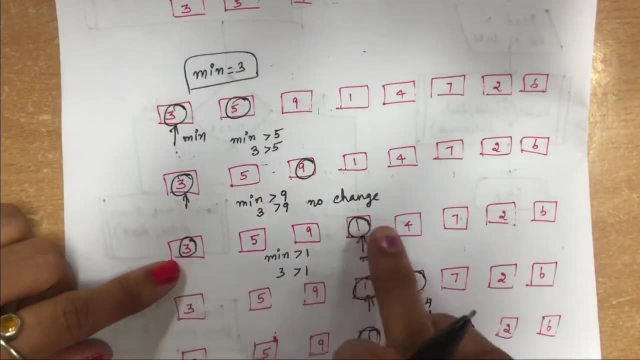 value. first, 3 and 5 is checked, so there is no change. 3 is smaller than 5. and again 3 and 9 is checked. 3 is smaller, so there is no change. 3 and 1 is compared. so when 3 and 1 is compared, 3 is the. 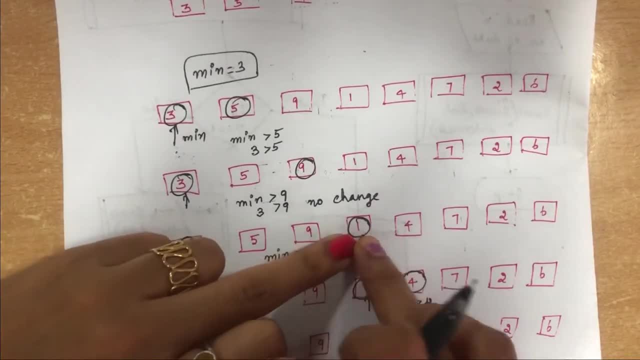 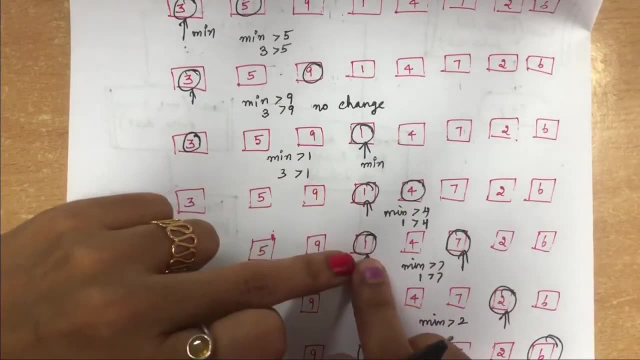 greater value than this 1, so i have to set this 1 as the minimum value. now i am going to compare this 1 with 4. when i am comparing 1 and 4, 1 is smaller, so i have to leave as it is. 1 and 7: 1 is smaller, 1 and 2- again 1 is smaller. and last, when 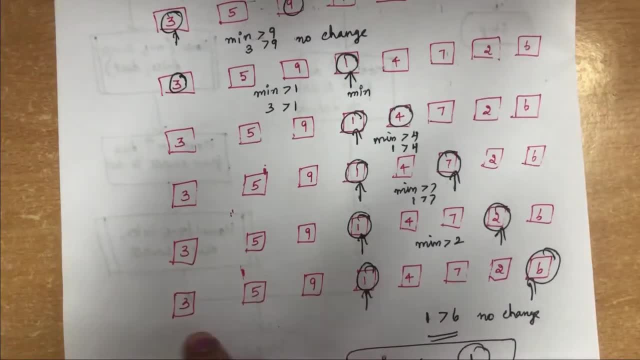 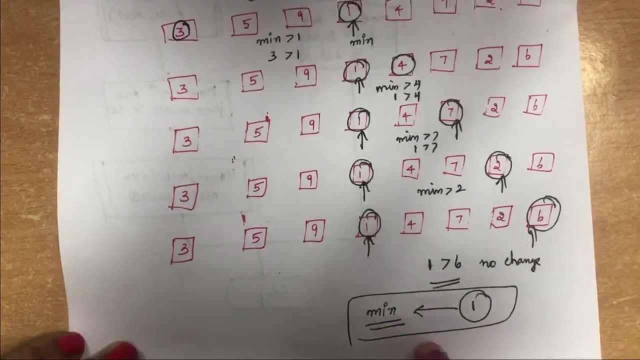 i proceed this: 1 and 6. again, 1 is smaller. so when i come, when i have checked this, all the list of numbers, i found that 1 is a smaller number among all the numbers. so this is will be considered as the minimum element in the particular list. so the same procedure. i am going to compare this 1 with. 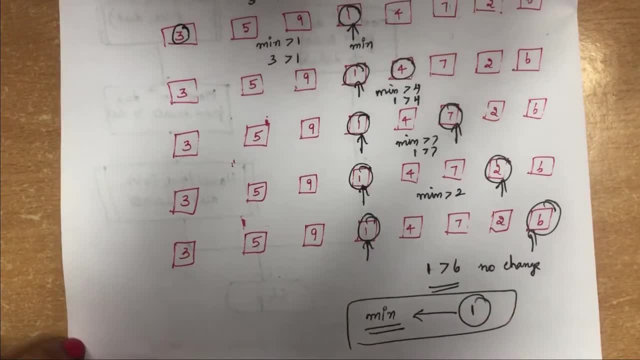 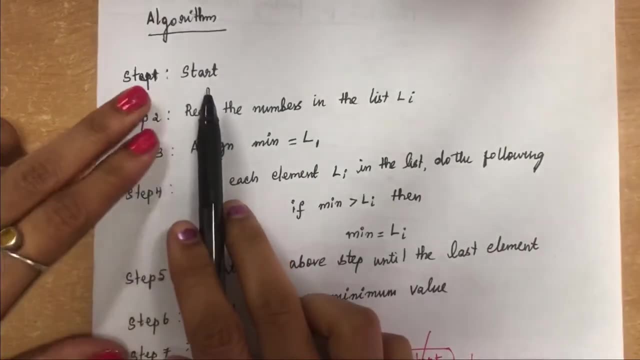 going to use it for implementing algorithm and flowchart. i think you all have understood this: finding the minimum in the list. now we see the algorithm and flowchart. the first step is start. the second step: i am going to read the list, so i am going to store the entire list in. 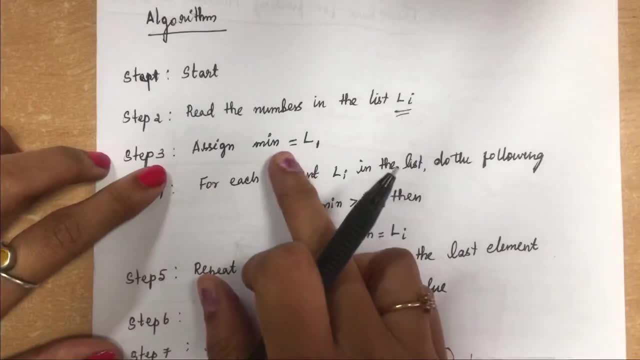 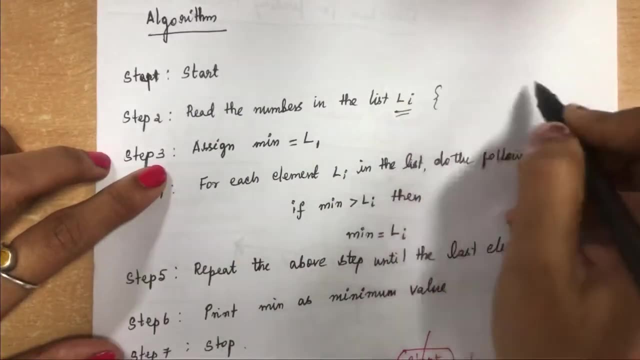 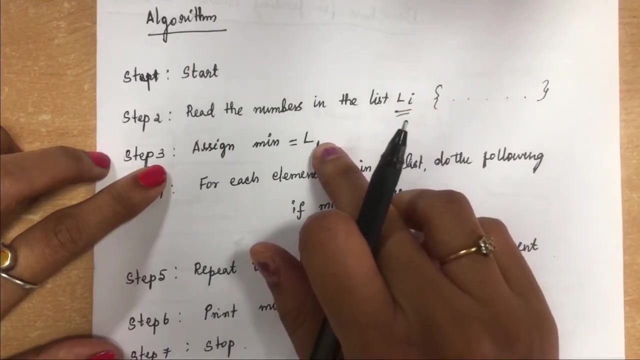 li. okay, the third step. what i am going to do is i am going to set the first element in the list to be minimum l1. so i have some set of numbers. i will get all the numbers over here. i am going to store it in li and in the first li that means l1 will be considered as the minimum element. that 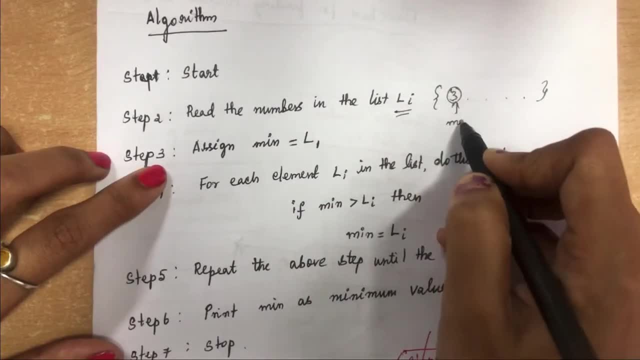 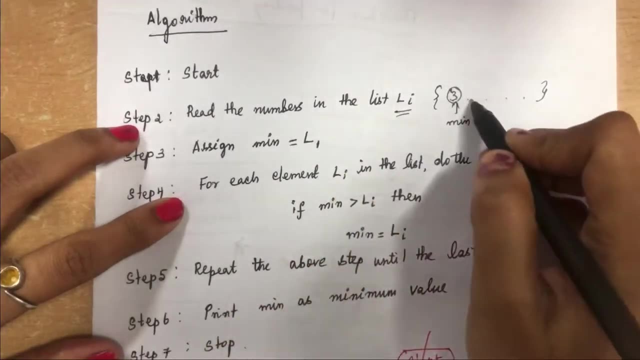 means the first element here. 3. this will be considered as the minimum element. okay, next the step. 4. i am going to use for loop for each element in the list, for each element in the list, do the following: i am going to do the two steps, the first step. what i am going to do is i am going 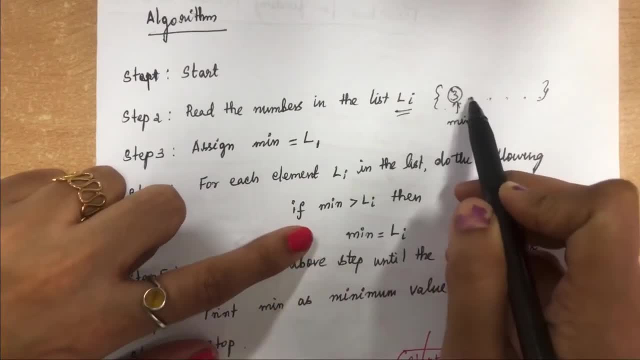 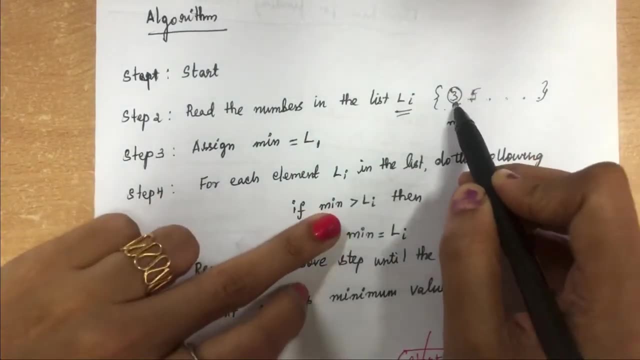 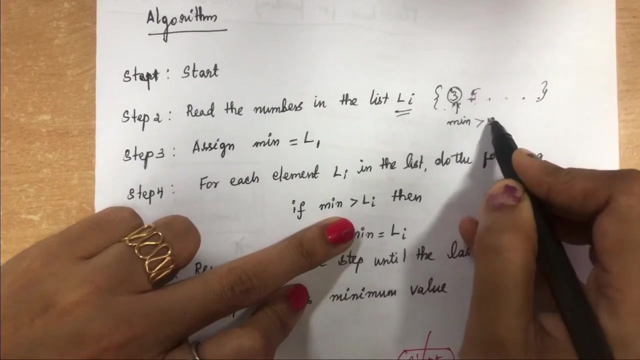 to check whether this minimum value is greater than the next element. suppose i am having this program. what i have considered is 3, 5, right? so i am going to compare this minimum element with the next element. so if minimum is greater than li, so if minimum is greater than 5, if the condition 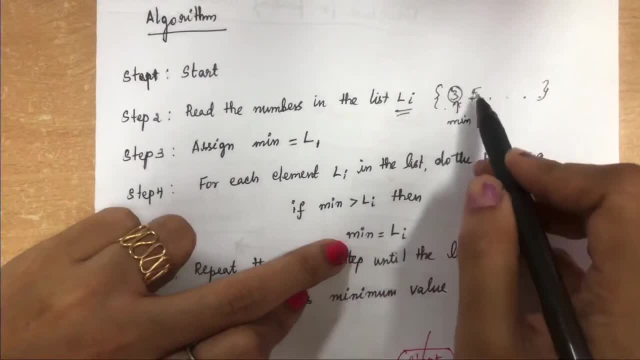 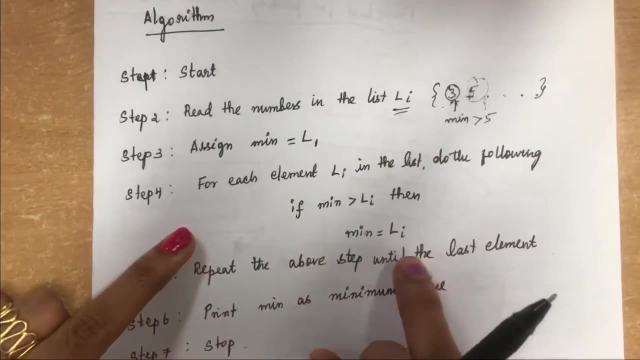 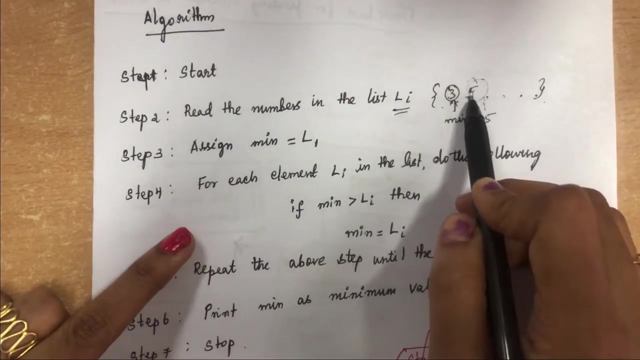 satisfies, then i have to set this value as the minimum. so if the condition does not satisfy, it has to repeat this loop. repeat this loop until it proceed to till the last element of the list. then, if the condition satisfies, then i have to set the second element to be the minimum. minimum is: 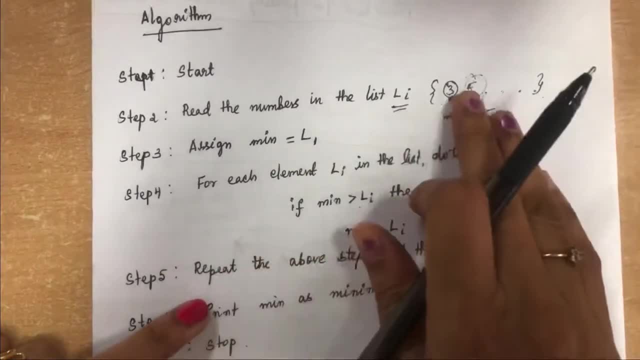 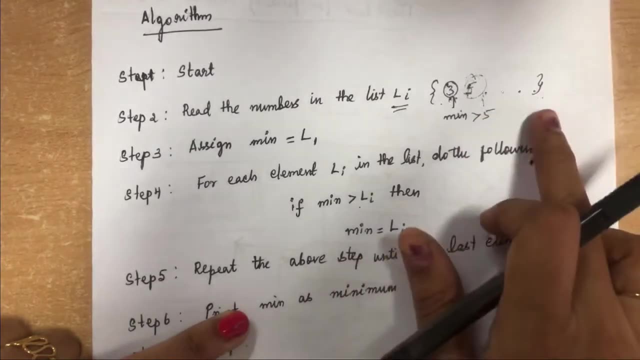 equal to li. so you have to repeat this. once i have completed traversing all the elements in the list, i can print minimum as minimum value which i have, which i will get at the end of the list, will be considered as the minimum value. so then i will stop the algorithm. okay, so what i am going to do. 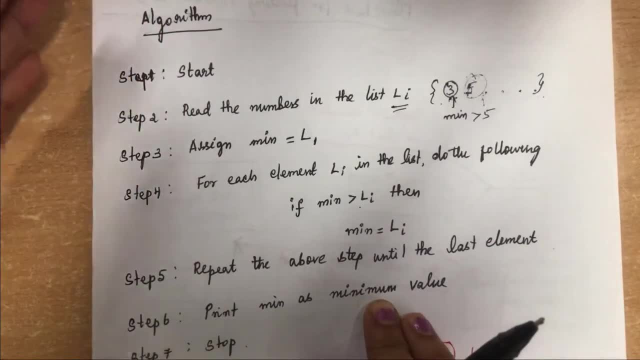 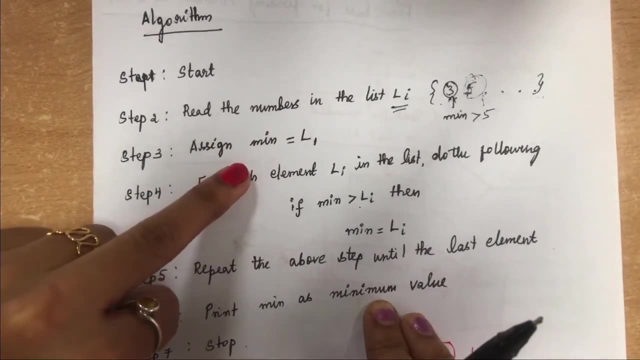 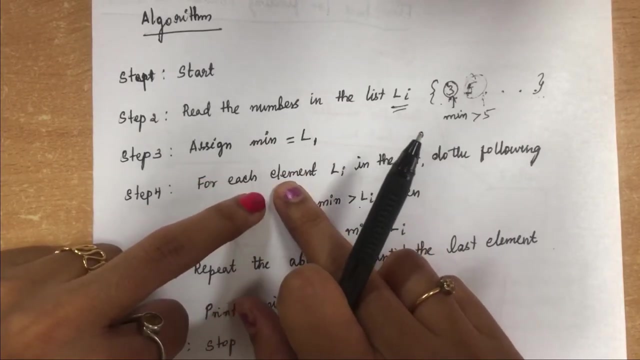 is the same procedure, what i have used for traversing, that i have implemented in algorithm. i have to read all the numbers in the list. next step is i have to set the first element to be the minimum element, so l1 to be considered as minimum. so i am using for element for loop to do the to. 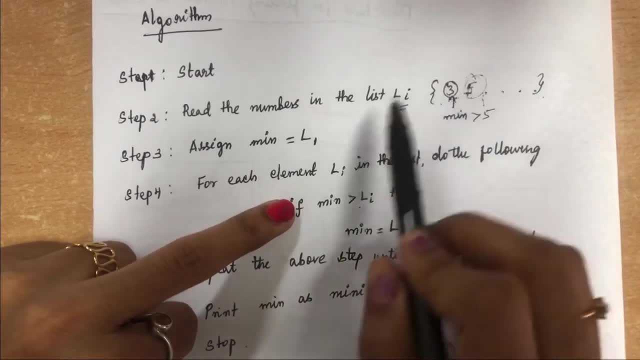 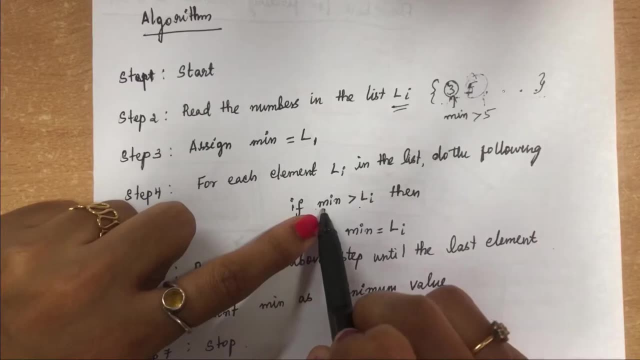 repeat the steps. so in that case, first i am going to compare inside the for loop i am having if loop. that means i am going to compare this first element with the next element. so minimum is greater than li, li means the next element in that list. so when i am comparing, when this minimum 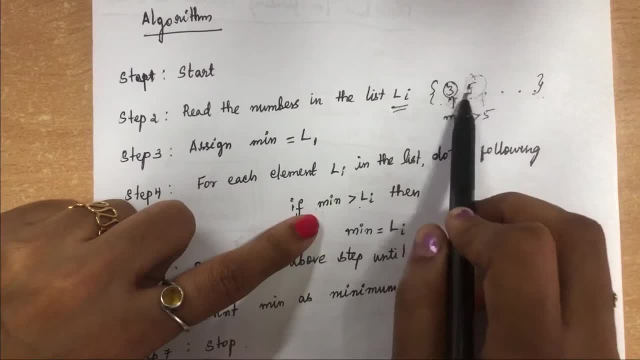 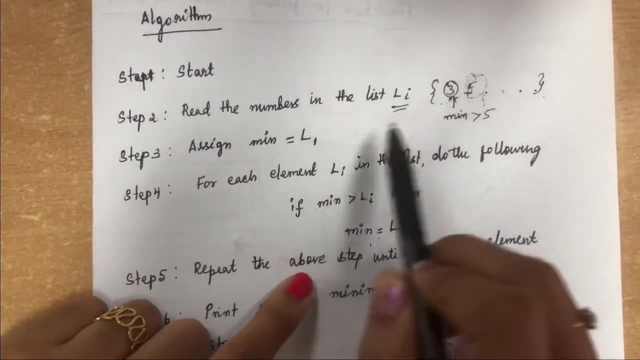 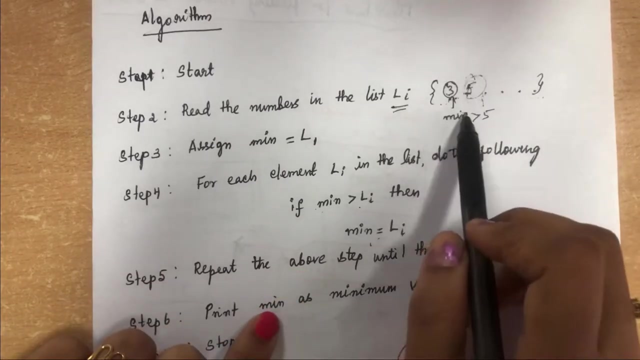 element is greater than li. that means the second element is the slower value. that means then i have to set this li to be the minimum value. okay, so this steps will be repeated until i am finishing all the elements in the list. once i have completed, the value which i have stored in minimum will contain the minimum. 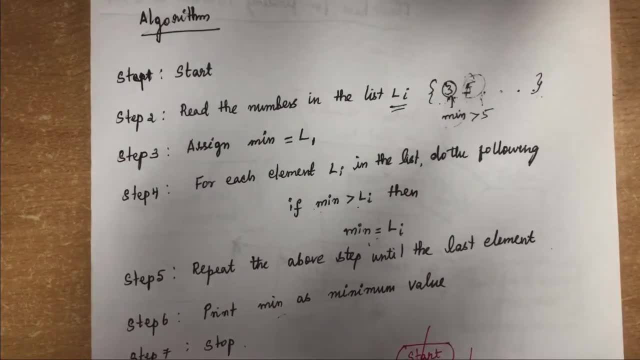 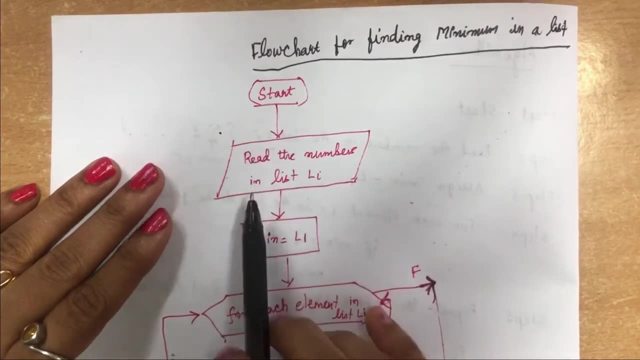 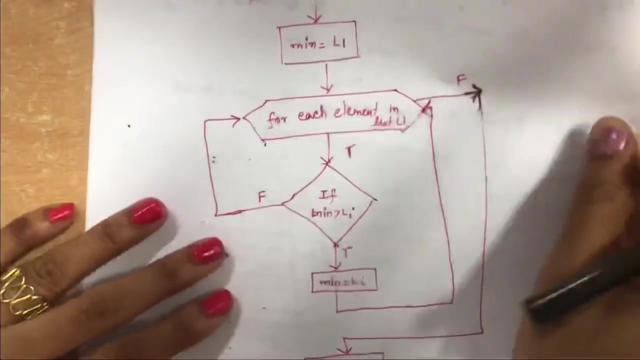 value. that is what i am printing it on the screen and i am going to stop the algorithm. now we will see the flow chart for this. coming to the flow chart for finding the minimum and list. so start read the numbers in the list. i am going to set the first element, l1, to be minimum for each element in the list, li if this. 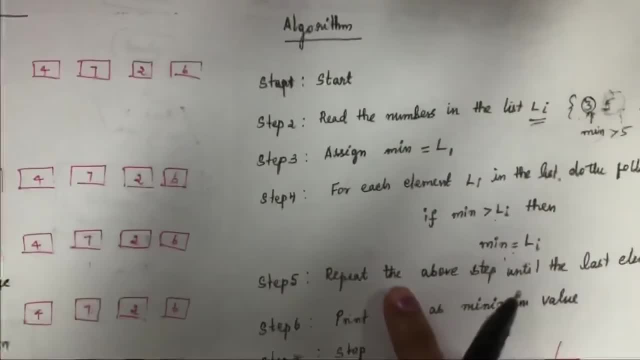 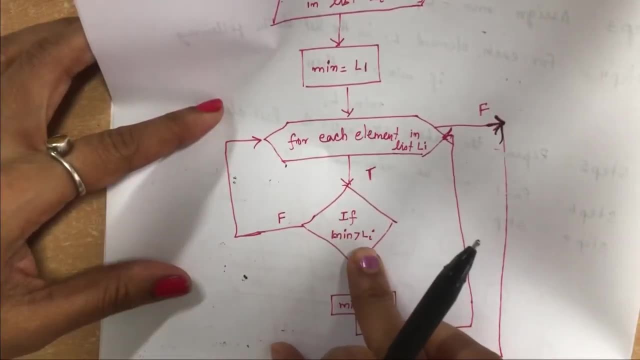 is true, i am going to check this condition. so in this case, i am checking the condition right. if minimum is greater than li, okay, so the same thing. i am going to do it here. if minimum is greater than li means true, means i am going to set that. next, the new value to be the minimum value. and again, 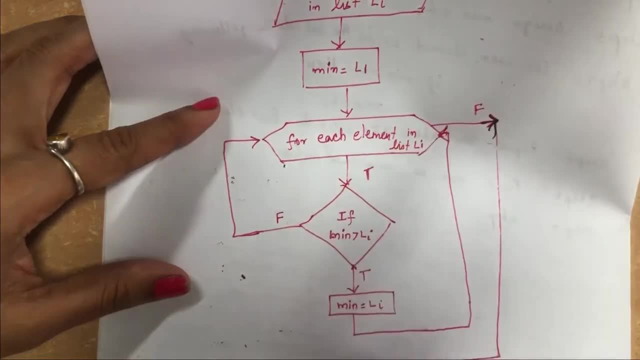 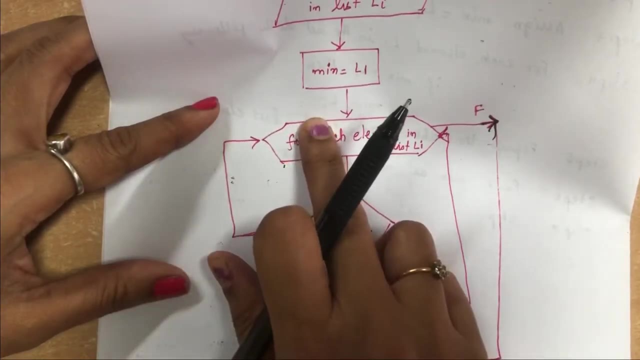 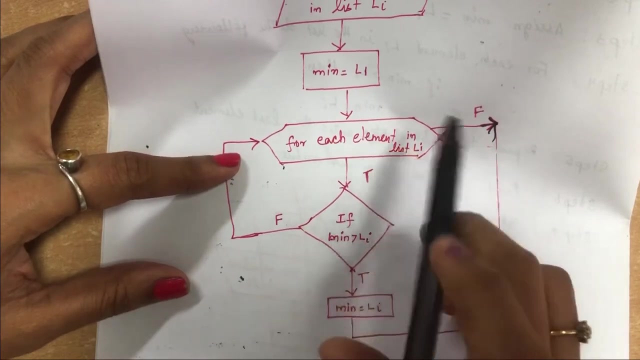 i am going to go to get the next element in the list. this process will get repeated, suppose. if this is true, okay, then it will come here and i will take the next element from the list. so this, these two will get repeated, suppose if i have traversed finishing all the elements in the list. 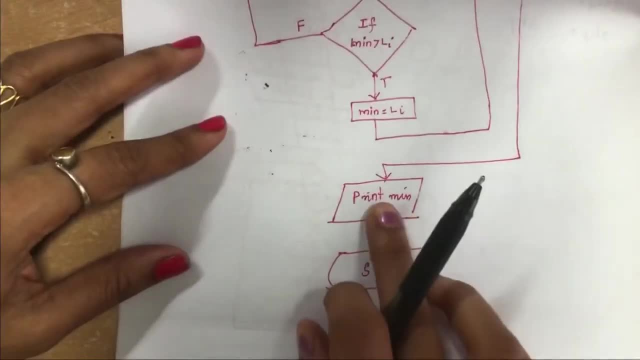 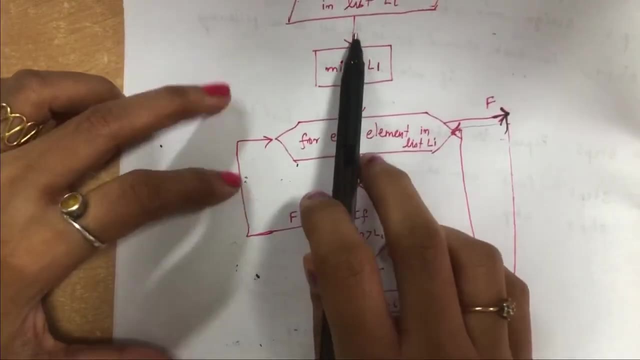 if this is false, then it will come here and go for printing the minimum value. then we'll go for stopping the algorithm, stopping the flow chart. okay, so first is that i am going to read the numbers, i am going to set this l1, the first element, to be the minimum value for every element. 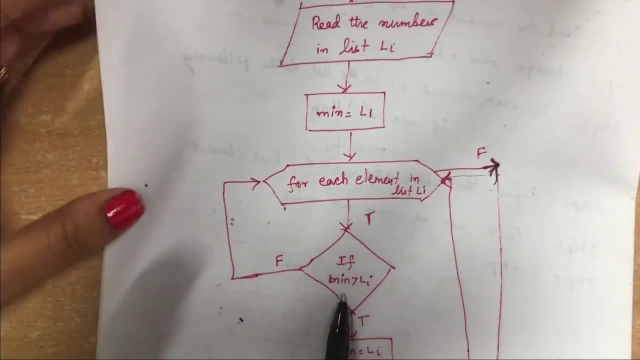 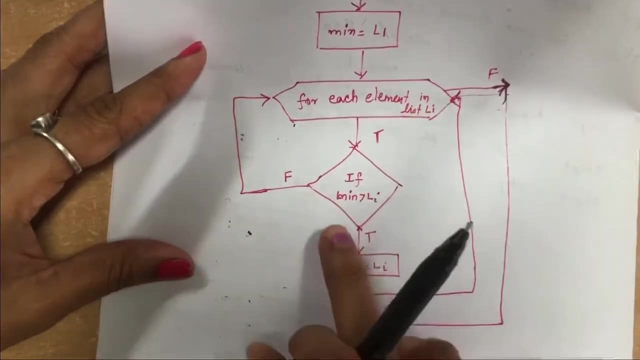 in the list. true means i am going to check for this condition. so i am going to check for this condition. if minimum is greater than li, then i have to set this new value to be the minimum value and i have to traverse this loop. if this minimum value greater than li is not, the condition becomes false. also, i 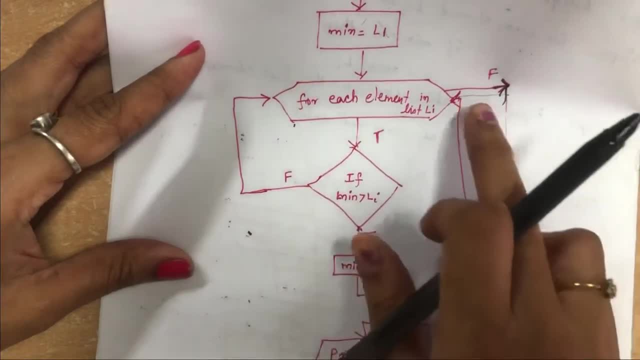 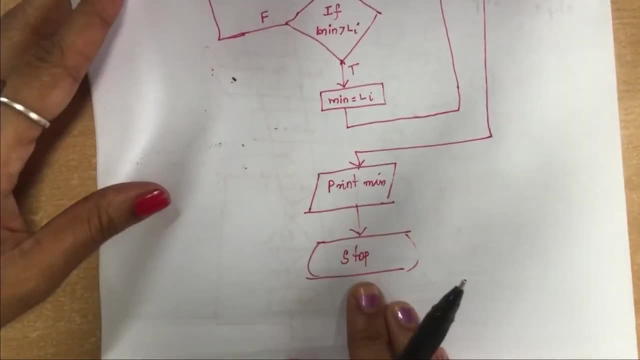 have to take the next element in the list and i have to compare. if this condition becomes false, it comes outside and it will print the minimum value. at last, it goes for stopping the algorithm. okay, the same process i am going to do. first. i am going to read all the numbers. 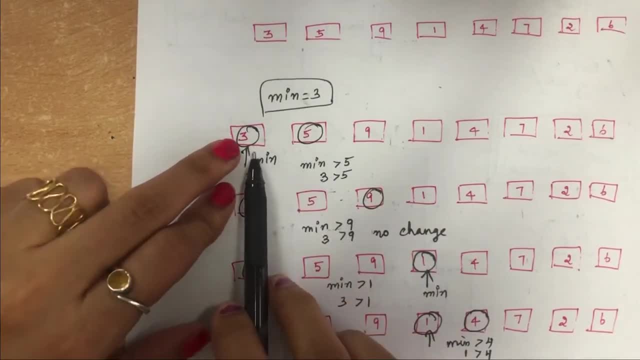 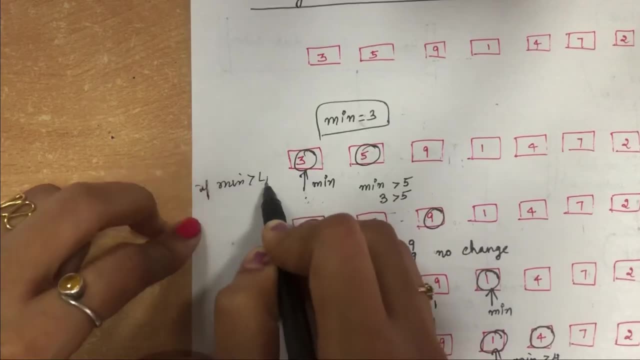 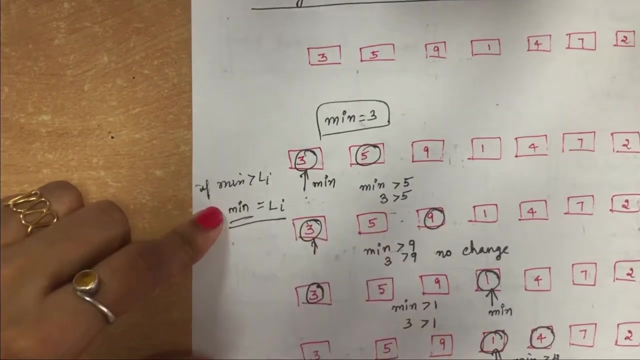 going to take for each element in the list, i am going to compare this minimum value with the next element, that is, minimum is greater than. if minimum is greater than li. if this condition satisfies, then i have to set this li value to be the minimum value. okay, this is the condition. 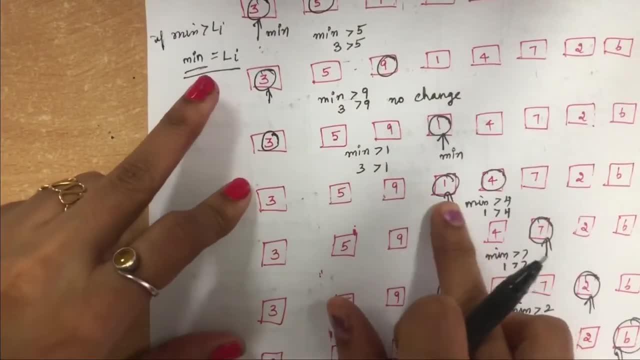 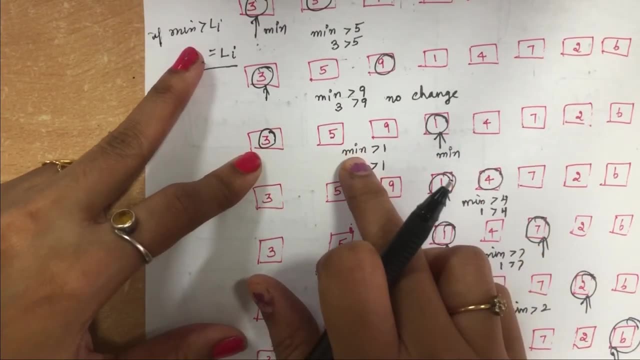 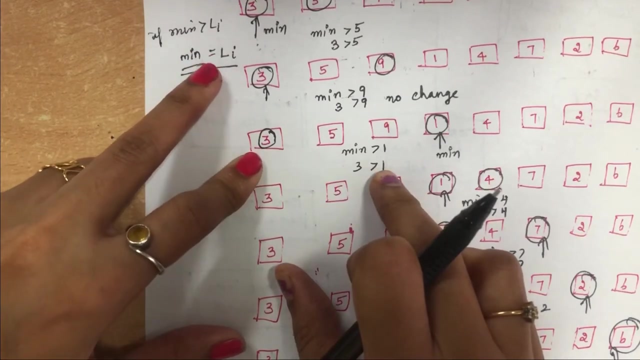 which you have to give it. that is why, in that case, in the, if you consider this case, if one and four is compared, suppose here three and one is compared. here minimum value is three and li value is one, so three is greater than one. if three is greater than one, what i have to?